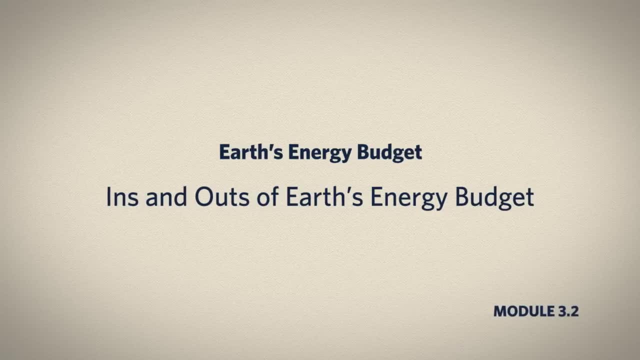 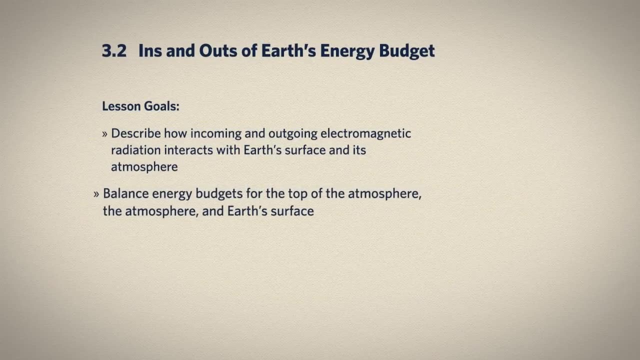 Hello and welcome to our introduction to Earth's energy budget and the various pathways by which energy gets transferred around in the system. Here's what we're aiming for in this lesson. There are a bunch of processes involved with energy in Earth's climate system. Some of them are super important, Some are slightly. 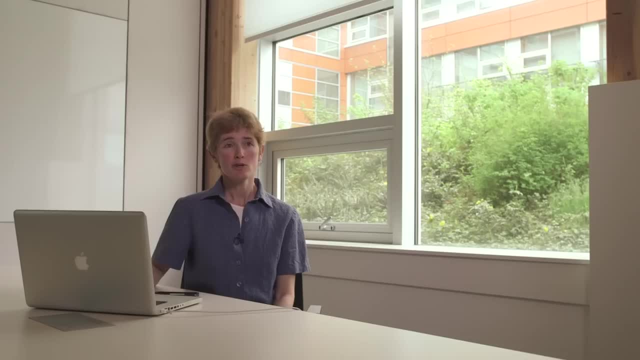 less important. But what is important is that you are able to describe some of the processes by which energy interacts with parts of Earth's climate system and get some practice checking for balance in energy inflows and outflows- Fundamentally, any mitigation actions we choose. 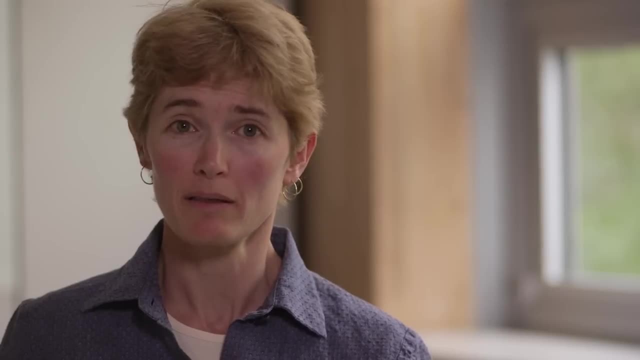 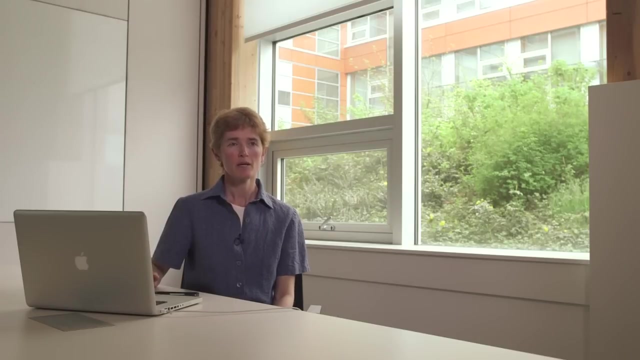 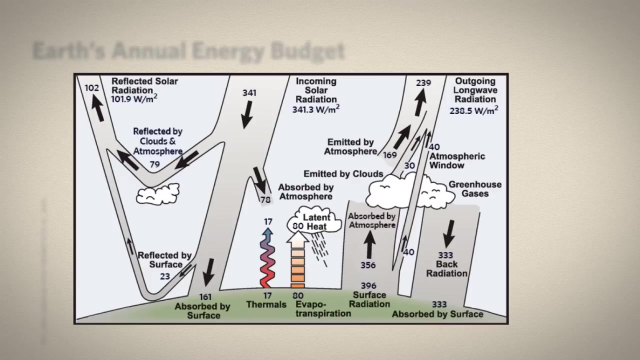 to take have to align with the energy flows we're talking about in this lesson. Where are the places we can actually do something to alter energy flows? Keep your eyes peeled for those opportunities throughout the course. We're going to spend this entire lesson focused on this one figure, which shows Earth's 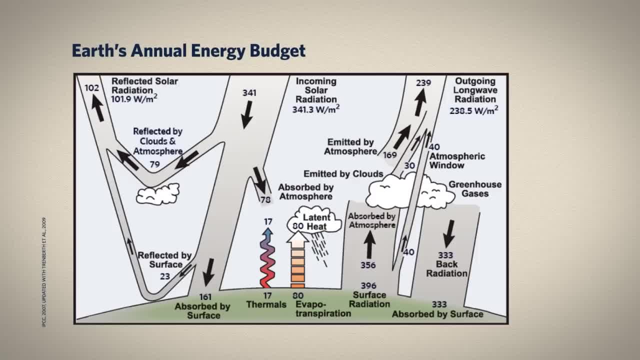 annual average energy budget: the energy coming in from space and leaving to space, The energy interacting with Earth's surface and the energy that interacts with Earth's atmosphere. There are a bunch of iterations of this figure. We're going to use this one. 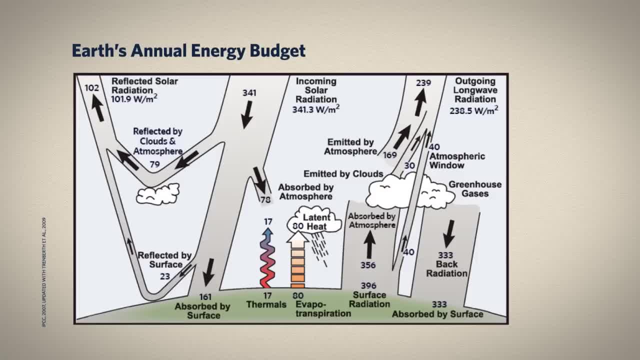 It's based on the IPCC 2007 report, updated with numbers from Trenberth and others from 2009.. Scientists continue to update specific numbers, but the important pathways are shown well here. All the numbers listed on this figure are in units of watts per meter squared. 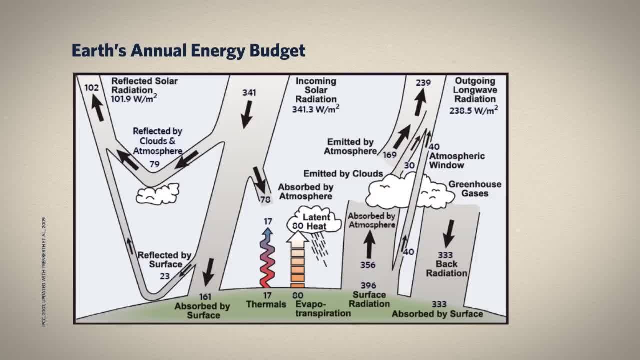 with which you're already aware that the energy flows from the Earth's surface are already familiar. We'll start working our way through this figure at the top, where solar radiation comes in. As we saw before, every square meter on the surface of the Sun emits 64 million watts. 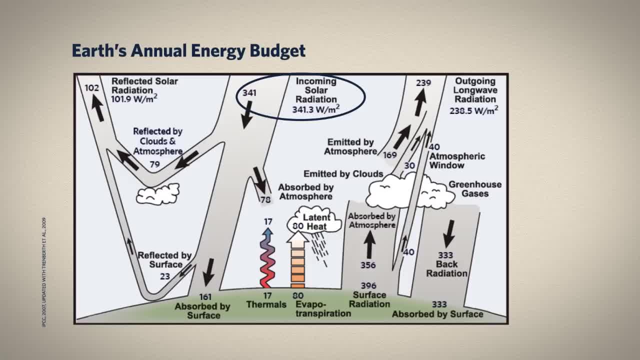 because the Sun is hot, That energy gets spread out over a bigger and bigger sphere as it travels away from the Sun, kind of like how the color of a brightly colored balloon fades as you blow it up bigger. By the time the Sun's energy has traveled to the Earth and 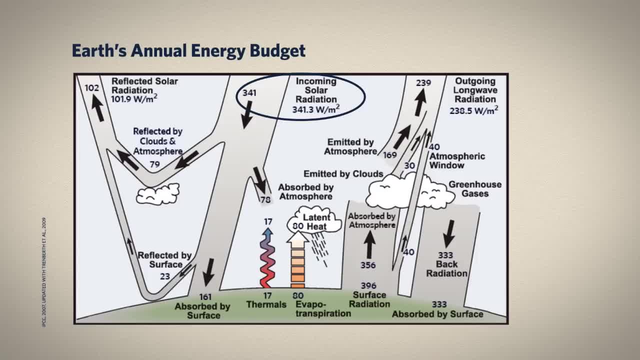 then, has been averaged out over our spinning spherical surface, we're down to about 341.3 watts per meter squared on average, for each square meter at the top of Earth's atmosphere. Remember that the type of radiation coming in from the Sun is centered at visible wavelengths. 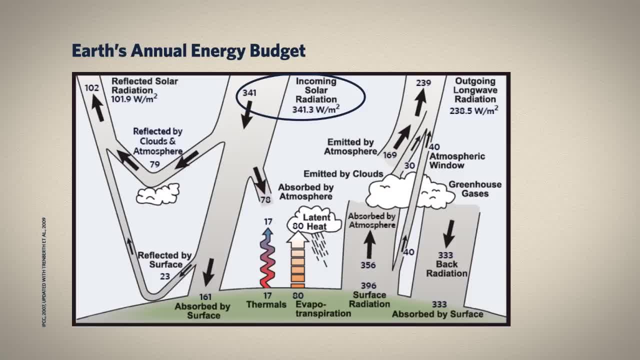 with some energy also in the ultraviolet and the infrared. Things happen to this shortwave energy when it encounters Earth's atmosphere. Some of this energy gets reflected back into space away, mostly by white things and shiny things in the atmosphere. White fluffy clouds are responsible for a lot of this reflection. 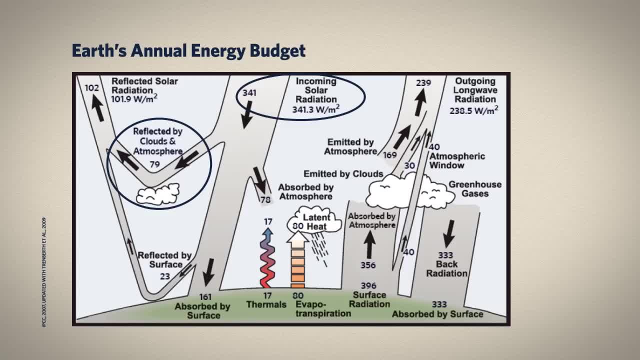 but there are also tiny particles in the atmosphere that act like little mirrors and reflect away some of than incoming radiation from the Sun. The atmosphere also absorbs some of the incoming solar radiation. Ozone in the stratosphere absorbs much of the ultraviolet on its way in and water vapor. is capable of absorbing a lot of it. The Crawl isonders light add up onto it, disrupting the radiation and blowing up the atmosphere. The particles are able to show a mixture of nice, absorbing some particular wavelengths of infrared radiation that overlap with the range of wavelengths 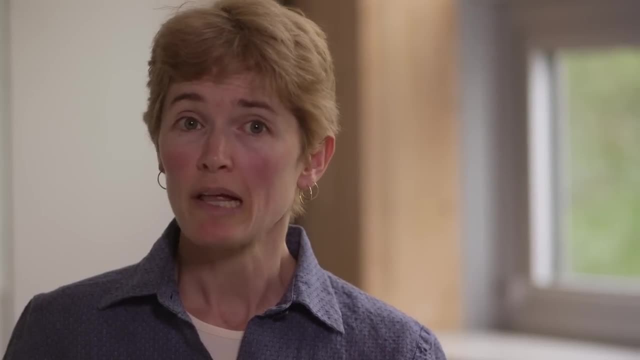 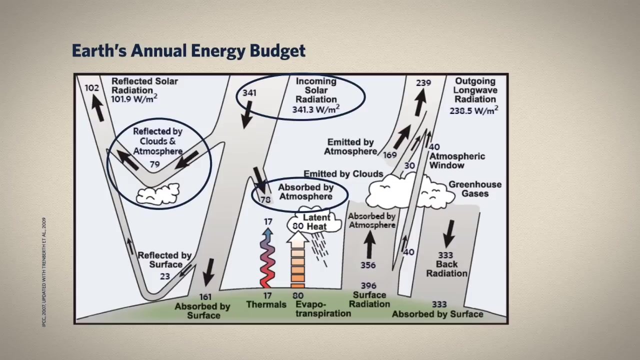 coming in from the sun. Dark particles in the atmosphere, like soot, can also absorb radiation. The atmosphere is mostly transparent to visible light, so a lot of the solar radiation passes through Earth's atmosphere and reaches Earth's surface. These are wavelengths that are mostly in the visible range and some in the infrared. 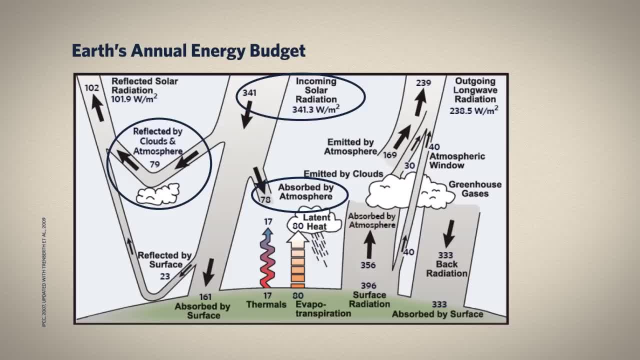 You can see two numbers that involve solar radiation reaching Earth's surface. On the left we have 23 watts per meter squared reflecting directly back to space. The surfaces that are good at reflecting this radiation are things like ice and light-colored deserts. 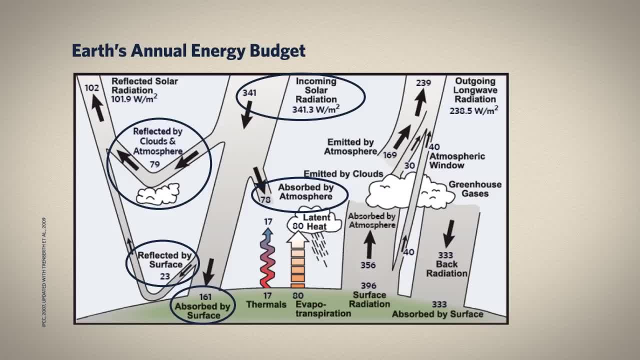 And 161 watts per meter squared are absorbed by Earth's surface. Notice that if we add together the solar energy directly reflected by the atmosphere and the solar energy directly reflected by Earth's surface, the two together would be the solar energy directly reflected by Earth's surface. 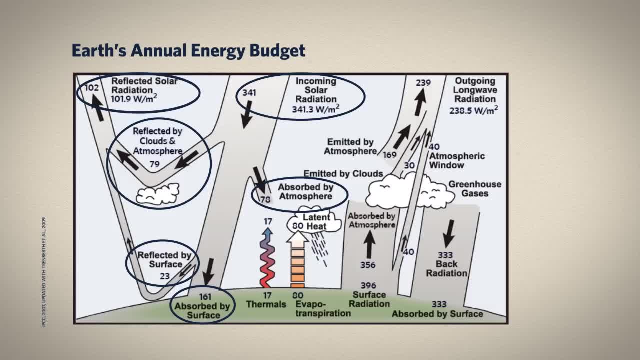 The two together would be the solar energy directly reflected by Earth's surface. These two together add up to about 102 watts per meter squared, So about 30% of the incoming solar radiation is reflecting right back to outer space and not really getting involved for very long. 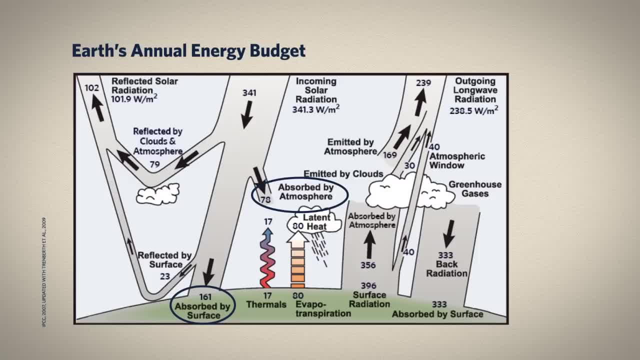 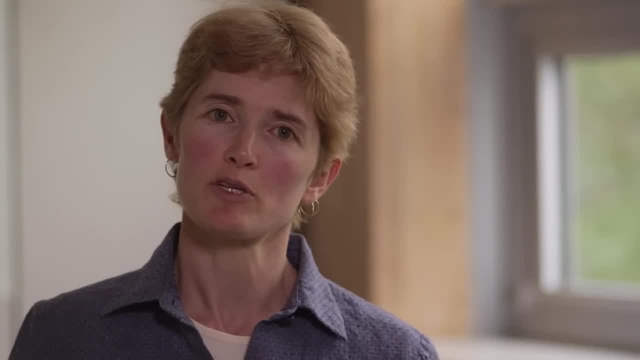 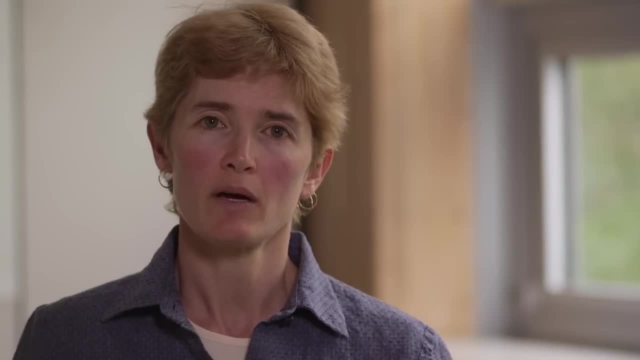 The other 70% is getting absorbed either by the atmosphere or by Earth's surface, for a total of about 239 watts per meter squared. Thinking from a systems perspective, what would happen if Earth's climate system continuously absorbed 239 watts per meter squared? 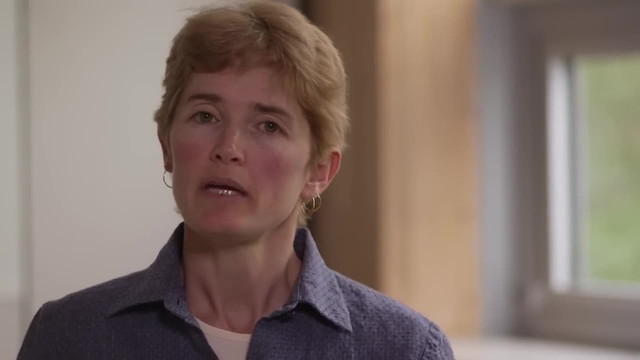 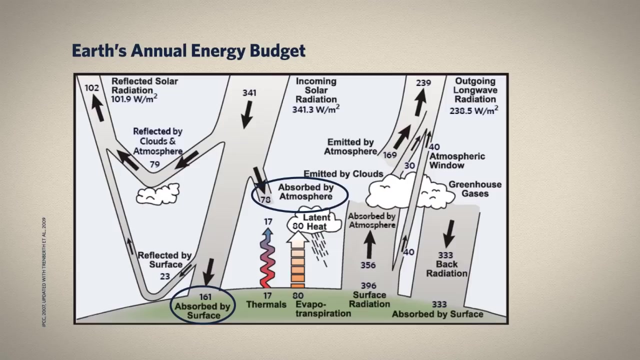 The planet's temperature would go up pretty quickly. But that doesn't happen because the planet also emits radiation back to outer space. so there's an outflow to compare to the inflow. If you look in the upper right you'll see that approximately 239 watts per meter squared. 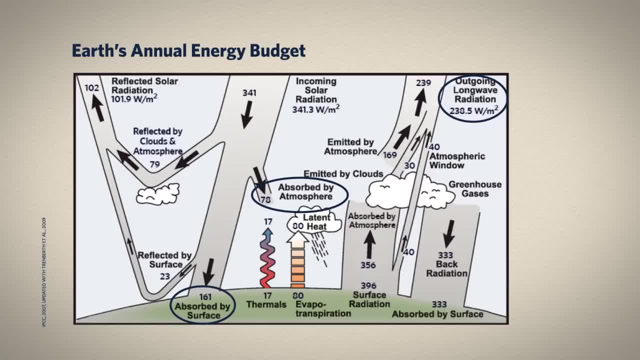 are ultimately leaving. as long-wave radiation too, Things get complicated. on the right-hand side of this diagram, We've seen that there's a lot of radiation in the atmosphere. We've seen that the Earth absorbs some energy from the Sun. This helps warm the Earth. 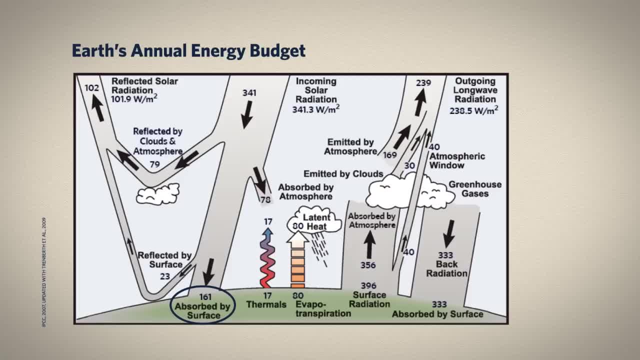 The Earth then, as an object at some temperature, also radiates energy, And it radiates infrared energy, long-wave energy, because it's a relatively cool object. That's the 396 watts per meter squared labeled surface radiation. A portion of that long-wave radiation, about 40 watts per meter squared, proceeds directly. 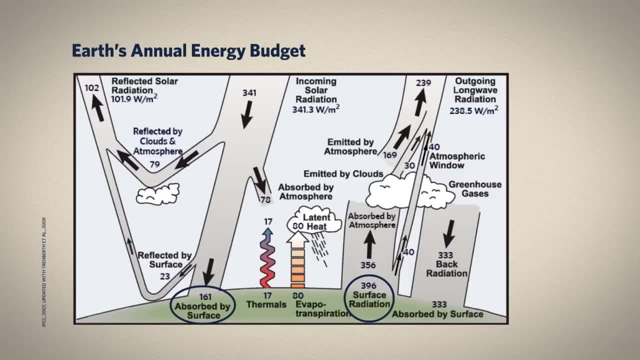 through the atmosphere to outer space. These are particular wavelengths of radiation that don't interact with any of the gases in our atmosphere, But a lot of the surface radiation doesn't make it directly out to space, but instead gets absorbed in the atmosphere by greenhouse gases and also clouds. 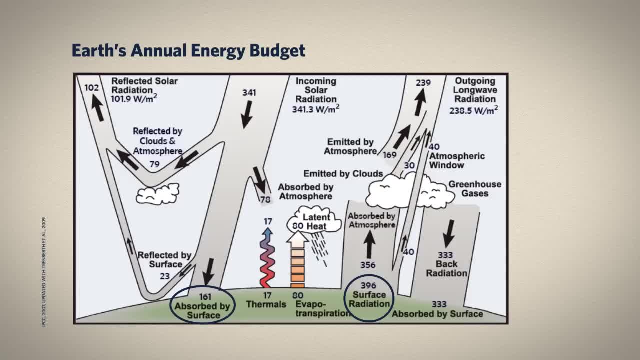 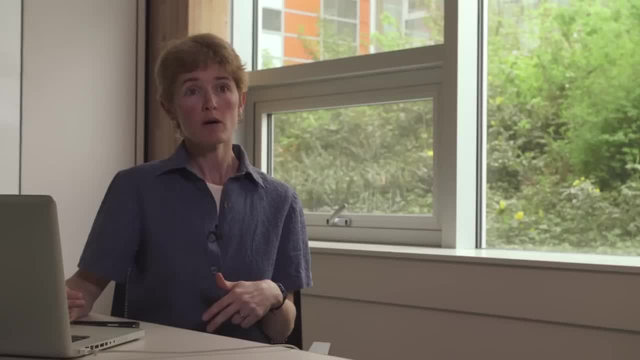 These then re-emit the radiation in random directions, though the randomness is not shown particularly well here, but it means the energy could go back towards Earth's surface, where it would get reabsorbed, helping to raise Earth's surface temperature, or the energy could go. 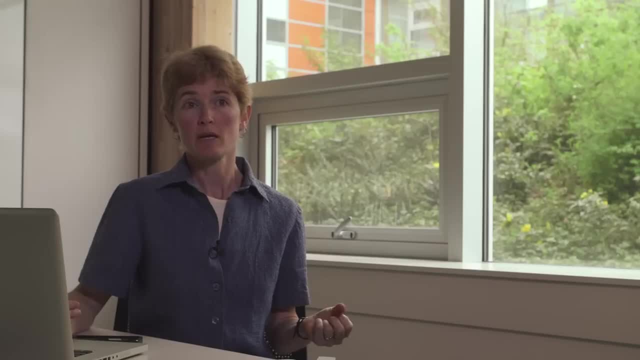 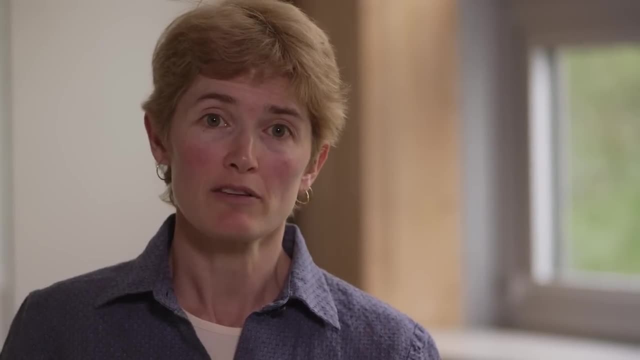 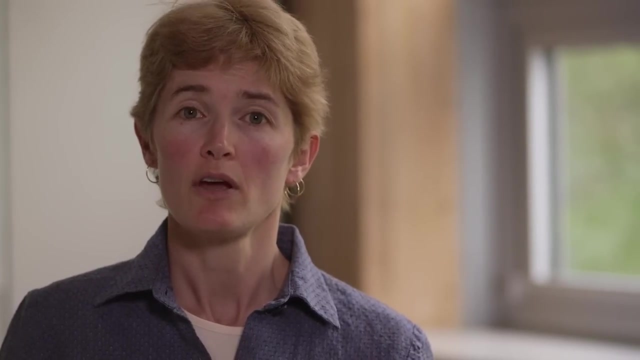 out towards space, or the energy could get absorbed by another greenhouse gas molecule, which will then re-emit it in yet another random direction. We'll look at more detail about the greenhouse effect in another lesson. The point here is that the presence of greenhouse gases slows the passage of radiation from 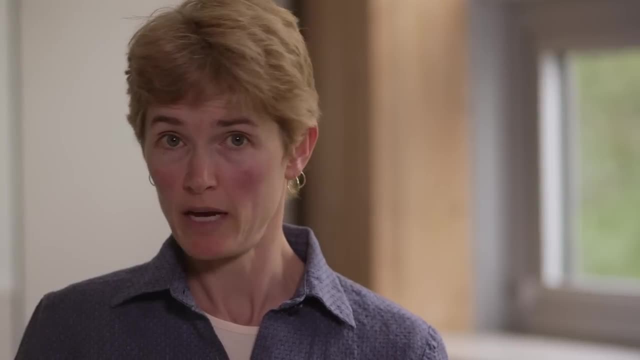 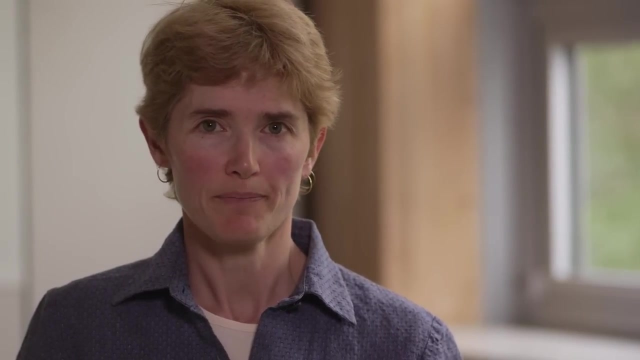 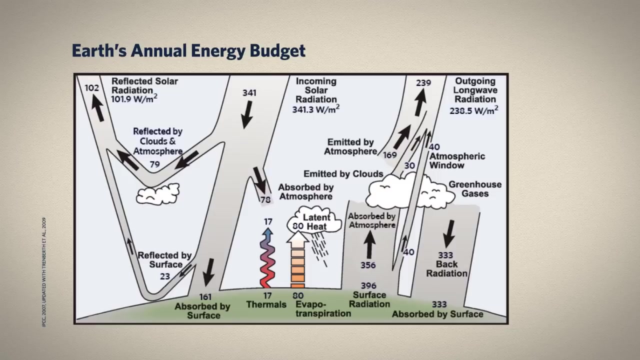 Earth's surface to space, increasing the total inflow of energy to Earth's surface, warming the surface which, as a now warmer object, radiates more energy. One minor point: Let's talk about energy balances. Most of the energy leaves Earth's surface via radiation, but some leaves via latent.